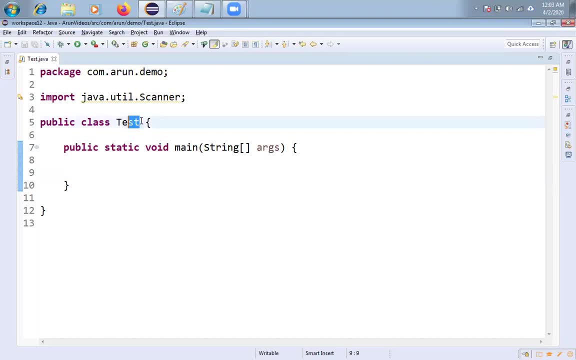 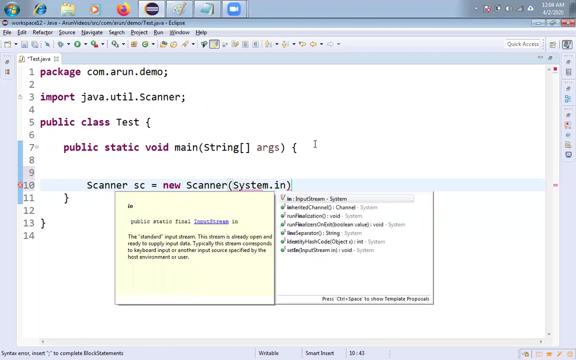 keyboard. so already i have taken one test class in that i have taken one main method. so let me create an object for one scanner scanner class. okay, and if you want to read any value from the keyboard, so you have to create one object for scanner class. so that's why- and i'm creating one object for scanner class- 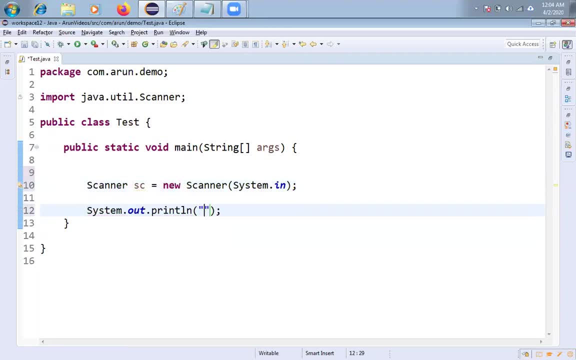 after that i'm trying to display one message on the screen, say: enter any two numbers i'm taking. integer a is equal to your c dot. next integer. integer b equal to your c dot, next integer. like first, i'll find common factors for these a and b. so that's why i'm taking one for loop and 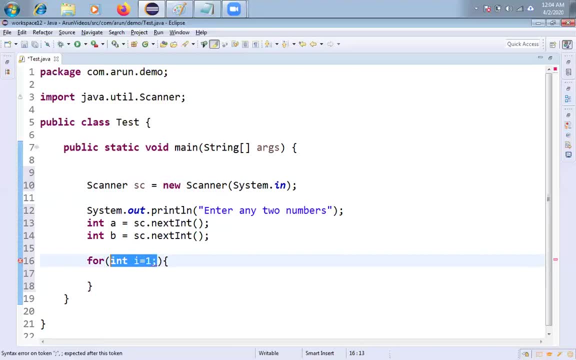 i equal to one. i mean why i am taking i equal to one is for any factor. i mean for any number factory, starting from one onwards. that is the reason i am taking i equal to one and i less than or equal to a also, you can take it, or b also you can take it. 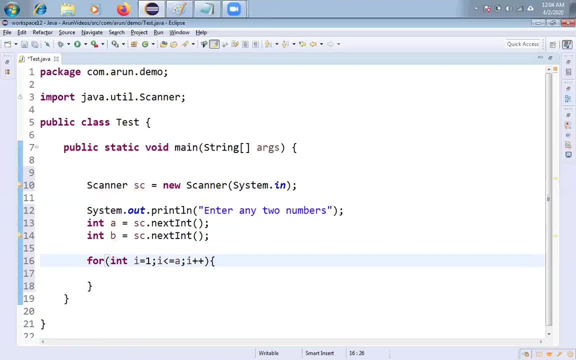 there is no issue. so i plus plus. so each and every number i will check first. i'll display all common factors. so for that one, i am dividing a with i and it should be zero. and i am dividing b with i and the remainder also should be zero. then i can say i is for. 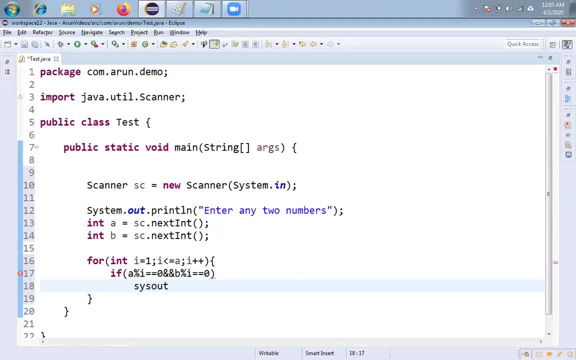 i is factor for both a and b, then i'm trying to display common factor. let me check it. i think in the previous video also we did it. but once again we are doing the same logic we are using for finding the common factors for, uh, given two numbers, say i'm giving 50 and i'm giving 60.. 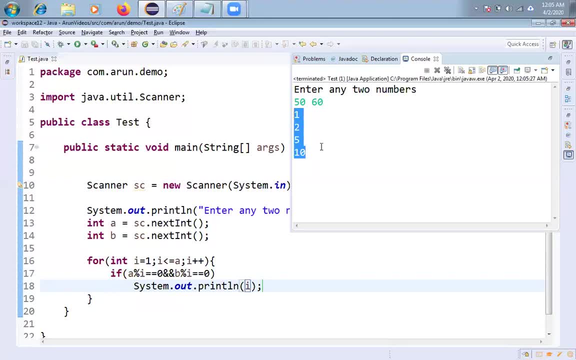 you are getting 1, 2, 5, 10.. so these are common factors. but i am not looking for common factors, i am looking for highest common factor, i am looking for greatest common divisor. so how to get 10? small thing, small logic? uh, very simple. i am taking one more variable. 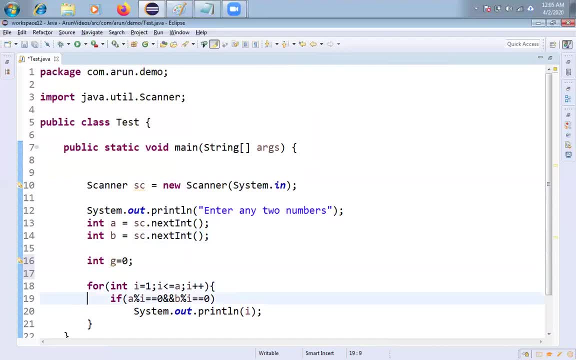 integer g equal to zero. okay, instead of systemoutprintln i am taking g equal to i. so what is the meaning? first time, what will be happen initially? g equal to zero, so i equal to one, so one, uh, i mean one divide, uh, i mean one divides a as well as b. so that's why what. 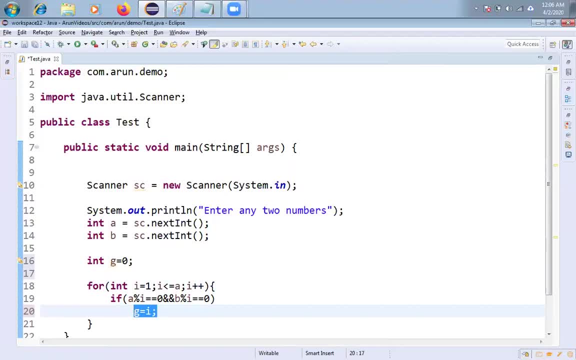 is the value of g, initially one, second time one will be. uh, like, i mean, one will be replaced by a, two, after that two will be replaced by five, and after that, finally, five will be replaced by ten. so the final value of g is ten. so that's why, finally, i am trying to display 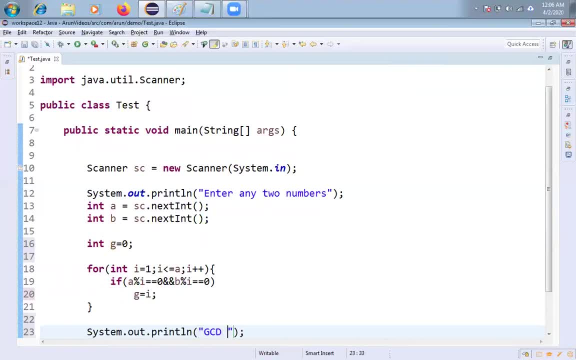 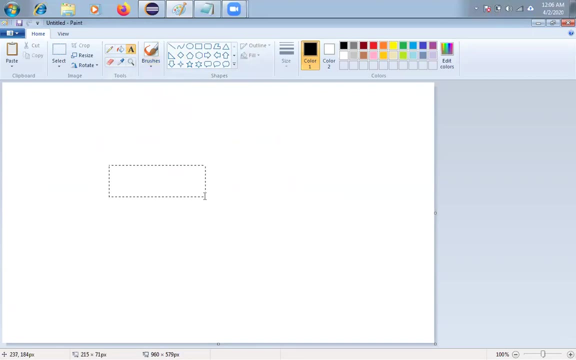 systemoutprintln gcd value. i'm trying to display. that's it. if you don't understand, i'll explain here. come here. and what are the factors of these things? so i have taken five, comma ten, sorry, fifty and sixty, a fifty and sixty, what are the common? 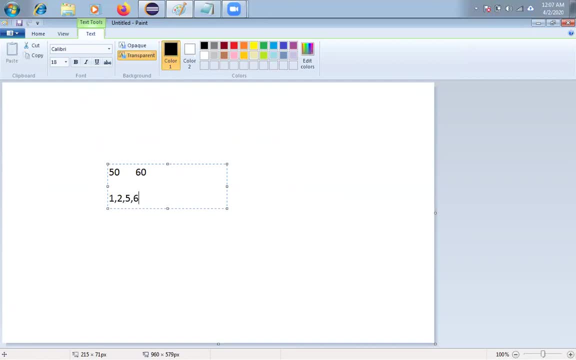 factors of fifty and sixty: one, two, five and ten. here i am taking integer. g equal to zero first time. what will be happen? g equal to one. second time, g, uh, second time, two will be coming. then two will be replaced by. i mean, one will be replaced by two. third time, five will come, so two will be. 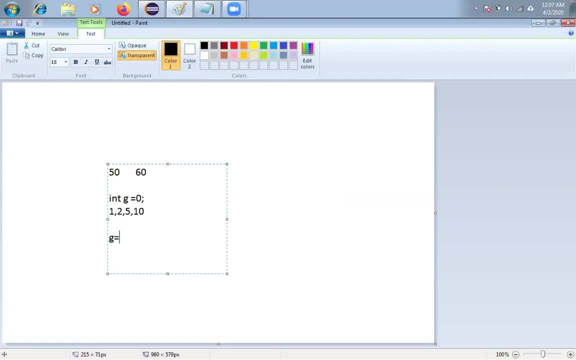 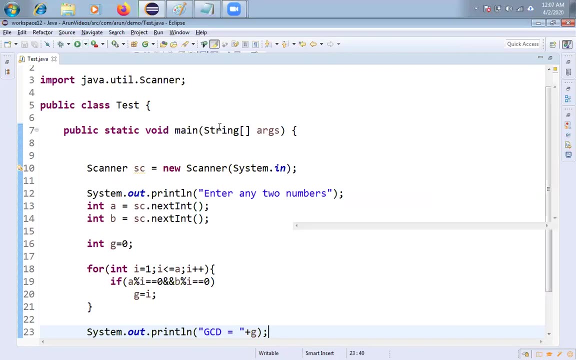 replaced by five. so finally ten will come. so five will be replaced by ten. so now g will be ten. so let me execute it, whether my logic is working or not, under any two numbers, 50 and 60, i'll get 10.. let me check it for one more set of values. i am giving 1000 and 2000. i am looking for 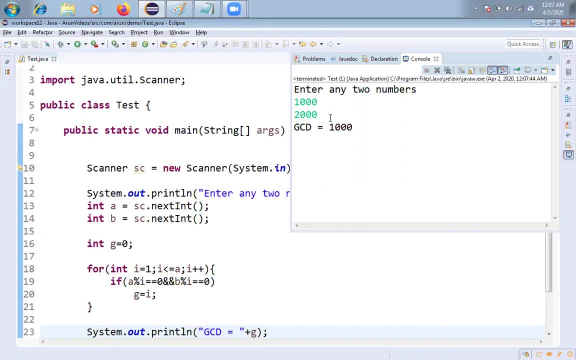 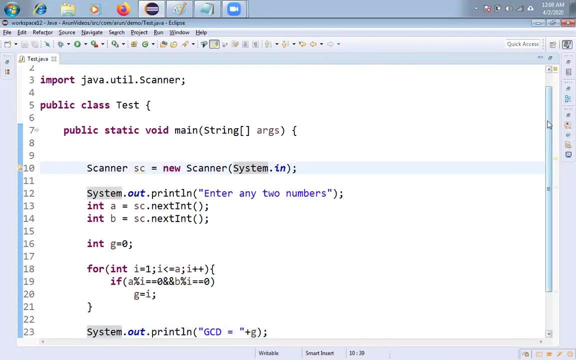 i want to find out gcd for 1000 and 2000. then what will be happen? gcd is thousand. let me check it for values. so that's why i am taking eight and nine. the gcd is one, okay, and in the next video. so what is the problem with this logic? uh, like more number of it will require more number of uh iterations.